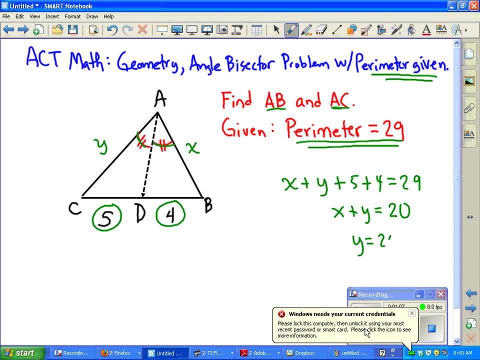 to 20, right, So Y is actually 20 minus X. So what we'd like to do is work with a single variable. So I'm going to replace Y with 20 minus X. So I'm going to say, instead of using: 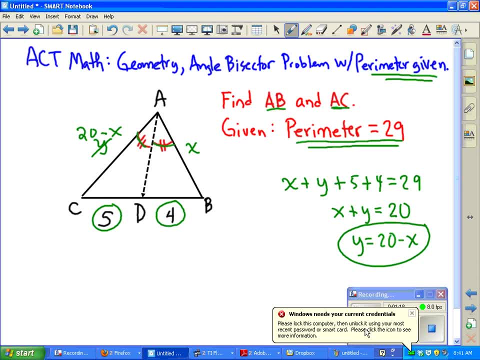 Y, let's use 20 minus X for this side. And so now what we have is we have a proportion. Using the angle bisector theorem, we know that this side here, 20 minus X, is proportional of 5.. 20 minus X is to 5, as this side, X, is to 4.. A little equal sign there. So we're going. 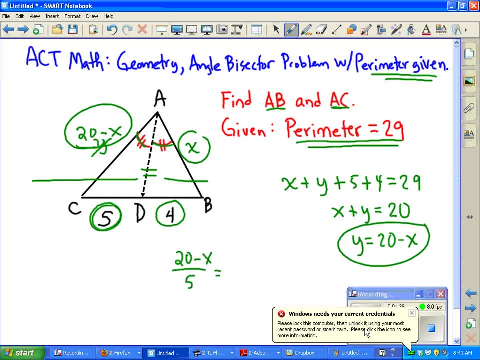 to say, 20 minus X is to 5, as X is to 4.. If we do a little cross product here, you're going to get that. Let me scroll down a little bit, Extend the page a little bit. You're going. 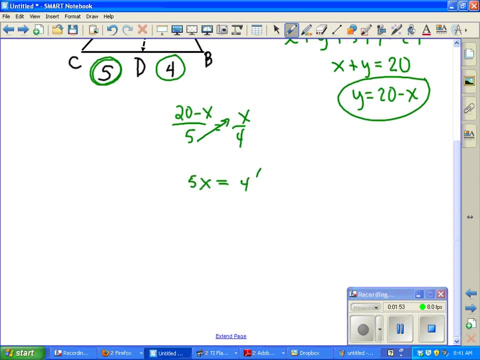 to get. 5X is equal to 4 times 20 minus X. And so if we use distributive property here, 80 minus 4X- that was equal to 5X. If you add 4X to both sides, 9X is equal to 80. And if you divide by 9, you're going to have that. 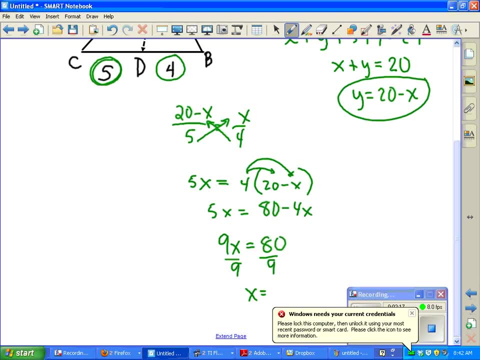 X is equal to 8 and 7 ninths, 8 and 8 ninths, or 8.88.. So let's keep it with a fraction, because we have to take that. Remember that one of the sides was X, The other one was 20 minus X, So Y was 20 minus. 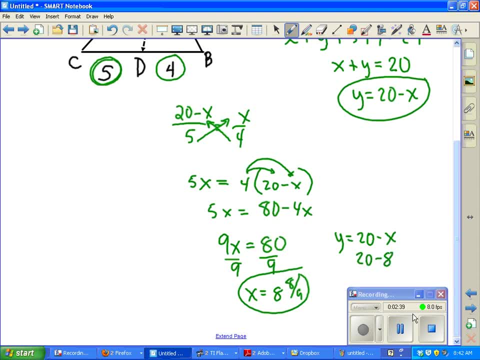 X, It was 20 minus 8 and 8 ninths, 11 and 1 ninth. Yeah, so 11 and 1 ninth, And these two 11 and 1 ninth and 8 and 8 ninths should add up to 20.. And so, therefore, we've got. 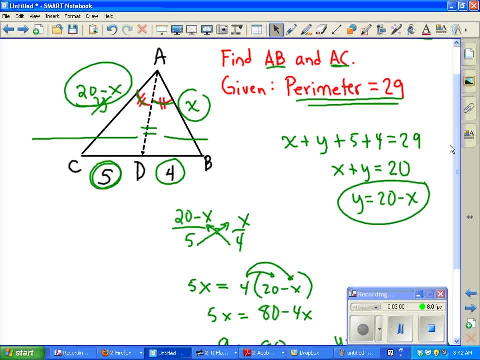 X and 20 minus X. So we now know that AB and we know what AC is. And those are the answers: 8 and 8 ninths and 11 and 1 ninth.